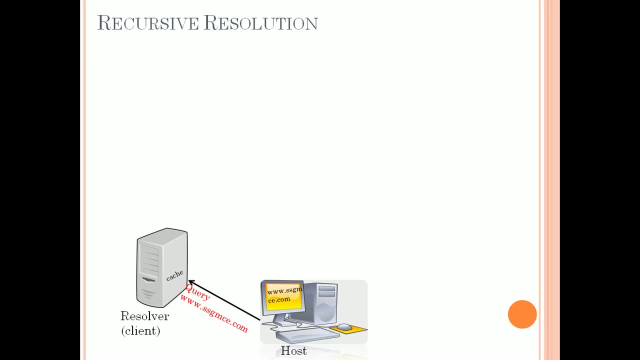 If it finds the IP address into its cache memory, it will send back a response. So the IP address is amount of 100,000 места. so its success is for a bot that is to provide these data to the hostiere. 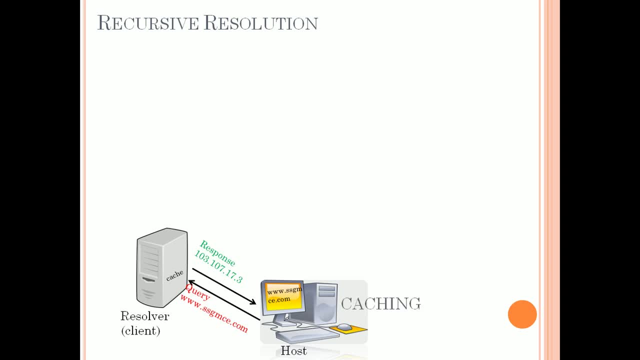 and it will redirect the IP address, making it go to resolution. This process is called as caching to the site. Friends caching is possible only when the host has accessed the site earlier. Friends caching is possible only when the host has accessed the site earlier. 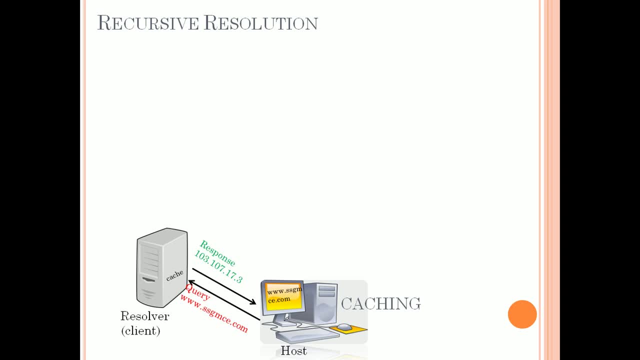 What happens in this is, if the native sites is in their home leven, the cancelation process is done from our server. in the other hand, this server of the Telfer connects to theenk server of the lambda we that we access the same websites. 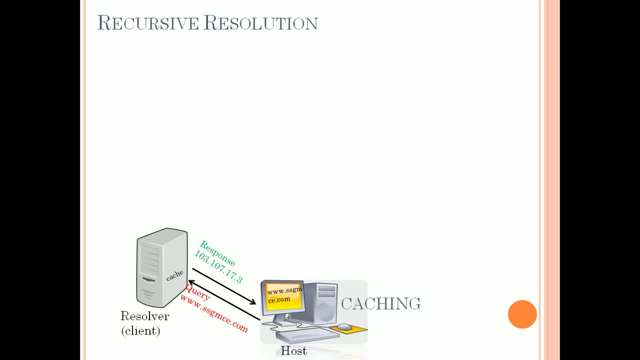 we can easily make this connection to it The same IP address. However, the caching is not possible if we are accessing the website for the first time. In that case, the response will not be available in the cache memory. So if you are accessing the website first time, the resolver will forward the query to the root server. 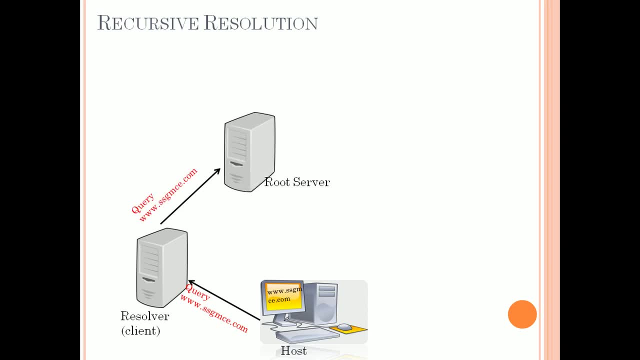 Now this root server will check the name, that is wwwssgmccom. In this the com represent that this query is of the com domain. So the root server will forward this query to a top level domain server. But which top level domain server? that is, your com server. 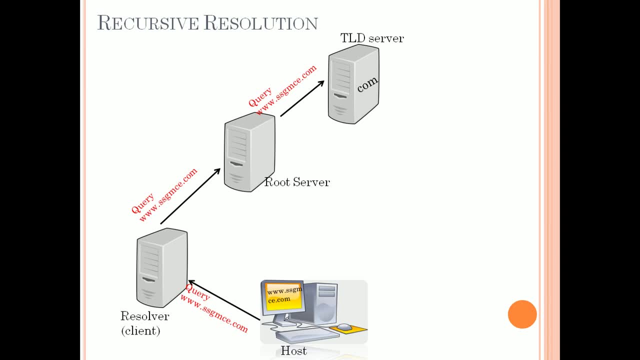 Now, when this query reaches the com server, The com server exactly knows which server is having the IP address, So it will forward the query to that particular server, Which is called as authoritative server. This authoritative server is the one which is having the actual table containing the mapping of names and IP address. 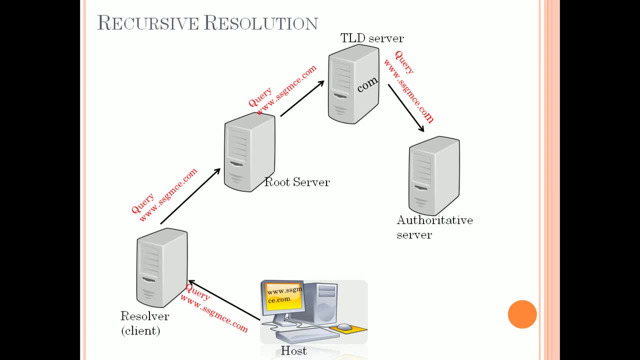 So the authoritative server will check the name, Will find out the corresponding IP address And will send back the response to the top level domain server. The top level domain server will forward it to the root server, Which will then forward it to the resolver And resolver will give it back to the host. 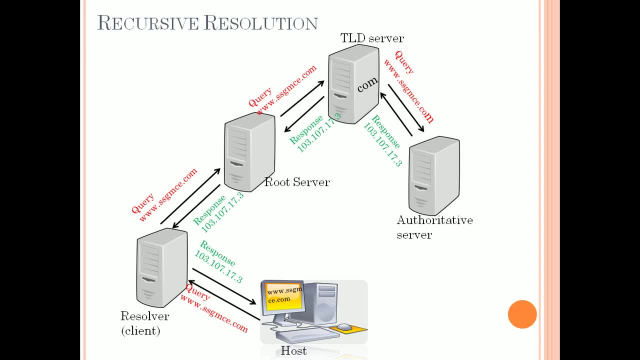 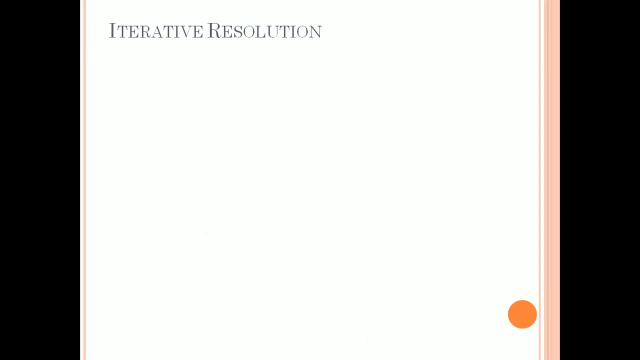 And also save it into its cache memory. So this particular process is called as recursive resolution. Friends, remember that in recursive resolution The resolver expects to get the IP address from the root server itself. Now let us see the next, that is iterative resolution. So again say, we are having a host that wants to access a website. 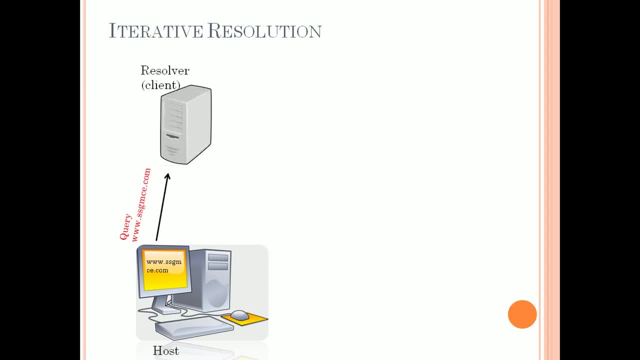 So the host will send the query to the resolver Again. the resolver will first check its cache memory And if suppose it finds the IP address, It will send back the response. The process is called as caching, as we already discussed. So, friends, caching is possible in both in recursive as well as iterative. 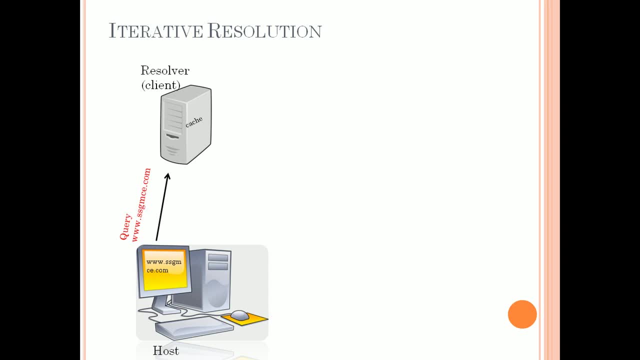 However, if it does not finds the response into its cache memory, Then it will forward the query to the root server. Now, this root server. what it will do? It will check again the name And it will find that it contains dot com. So, in this case, root server, in spite of forwarding this message. 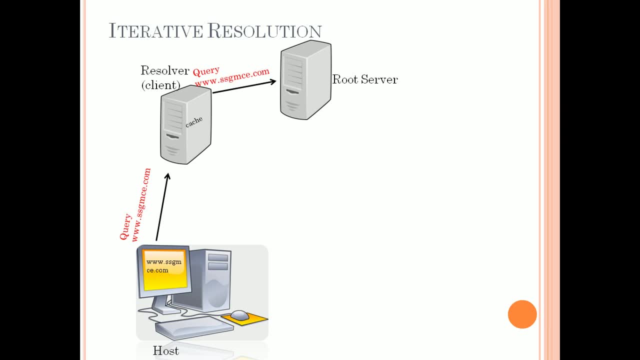 To the top level domain server Will send back the address of top level domain server to the resolver. Now resolver itself have to contact the tld server. So to contact the tld server obviously it will require the address of tld server. So resolver is having the address of tld server. 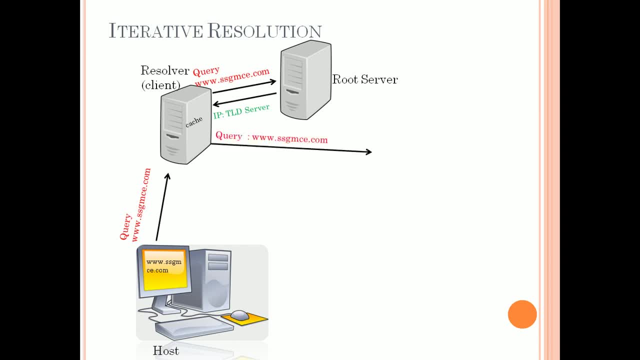 That it obtained from the root server. So resolver will now send the query to the tld server, That is dot com server in this case. Now this tld server knows which server contains the IP address for this name. Again, this tld server, in spite of itself contacting the authoritative server, 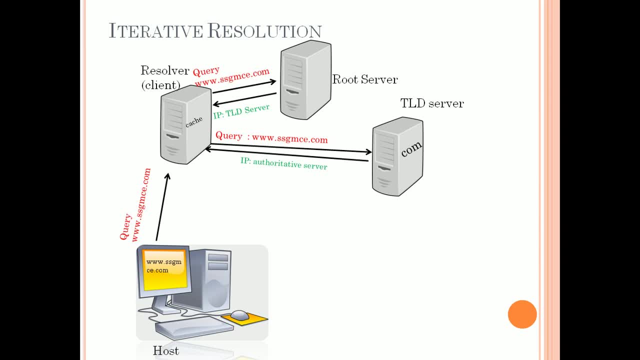 It will send the address of the authoritative server. Now again, resolver is having the address of the server which contains the IP address. Now resolver will send the same query to the authoritative server, Which is now the one which is having the IP address. So it will send back the response containing the IP address for that particular website. 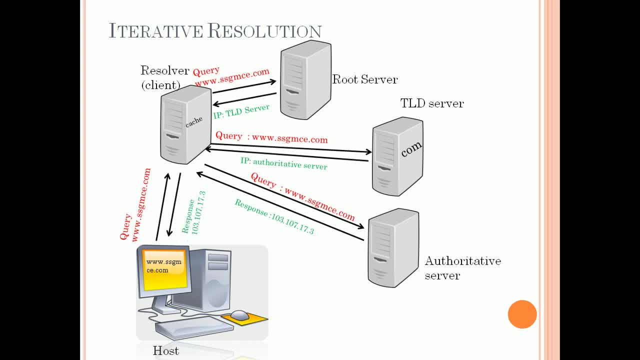 Now the resolver will save a copy into its cache And will send back the response to the host. So what happens in this? In this the resolver has to repeatedly send the request, That is, query message, to the different server. Hence it is called as the iterative type of resolution. 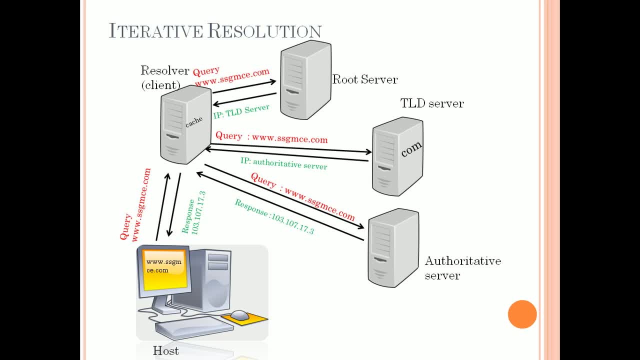 So, friends, this was all about recursive resolution and iterative resolution. For more videos on communication network, stay tuned with me. Thank you very much. 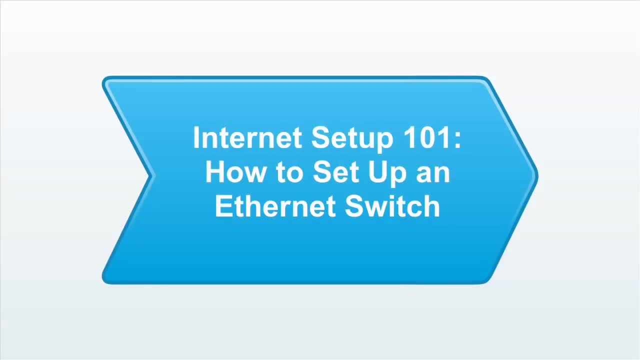 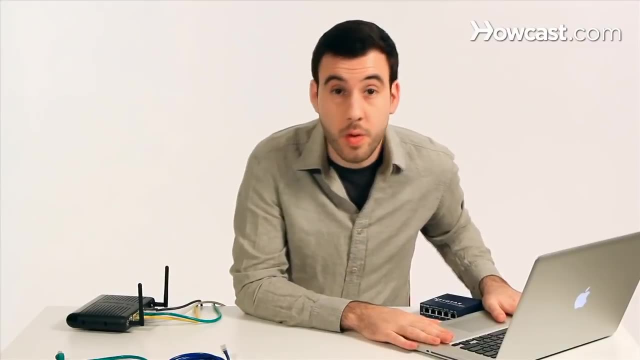 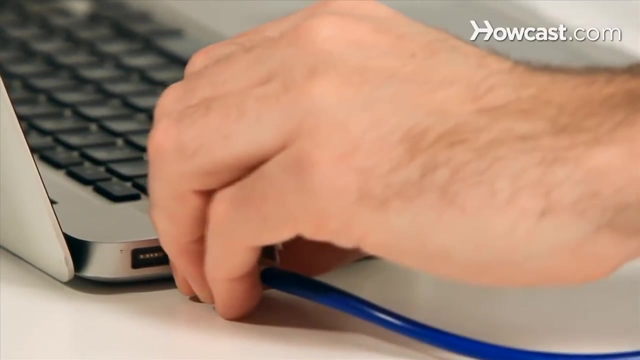 So in this video I'm going to talk about how to install your ethernet switch. So let's say I have my laptop here and I really want to connect it to my network, So I'll take a little ethernet cable and I'll plug it to the laptop And on the other side, of course, 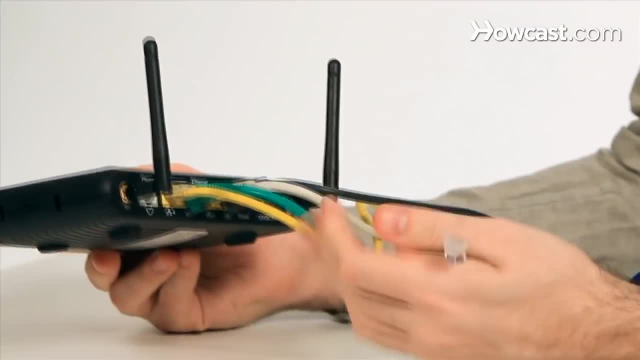 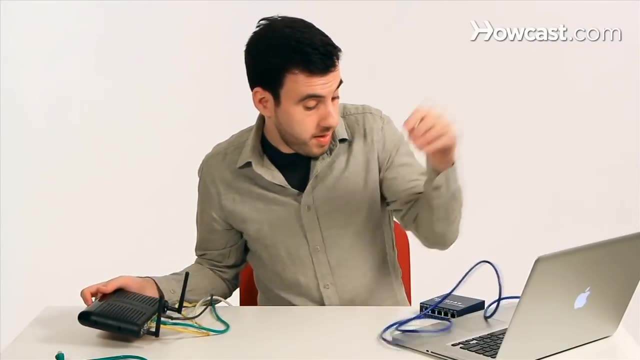 it has to go to my router. But oh no, I'm out of ports on my router. All my ports are already full because I've connected them to all my other computers. So what am I going to do? This is where the ethernet switch comes in handy. As you can see, the ethernet 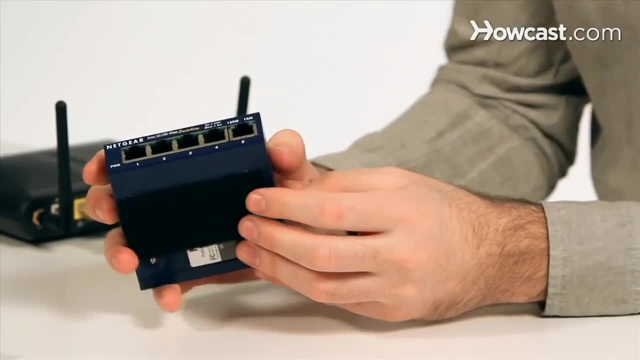 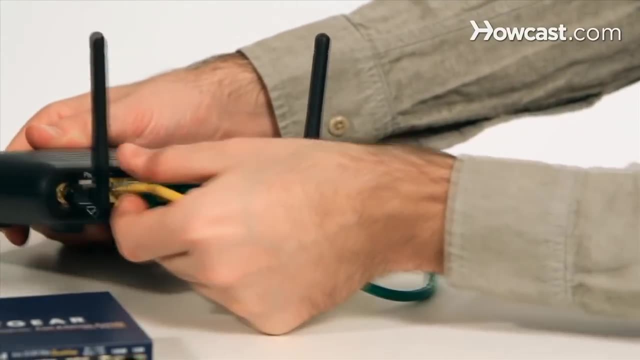 switch just has a bunch of ports on it, So to connect it to the network, what I have to do is first take one of the ports that are already connected to the network and move them over to the switch. Now, the reason I'm doing that is because I need a free port on 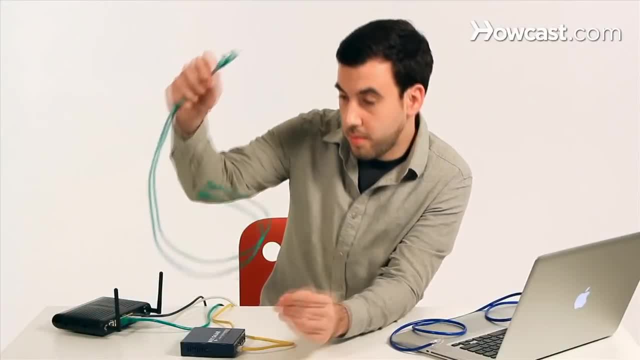 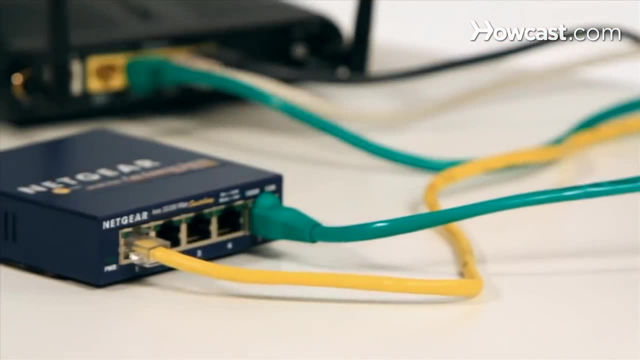 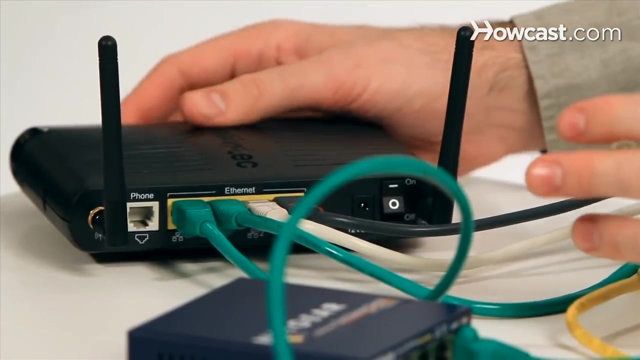 my router so I can connect my switch to. So I'm going to take another ethernet cable, plug that one in And then the other side goes to my router. Now it doesn't really matter where you connect the cables to. as long as the order is correct, The specific port is of no importance. So as long as I connected the switch to the router, everything that's connected to the switch is also connected to the router. Basically, the switch just extends the ports that are on the router. So now I have to just connect my laptop over to the switch. 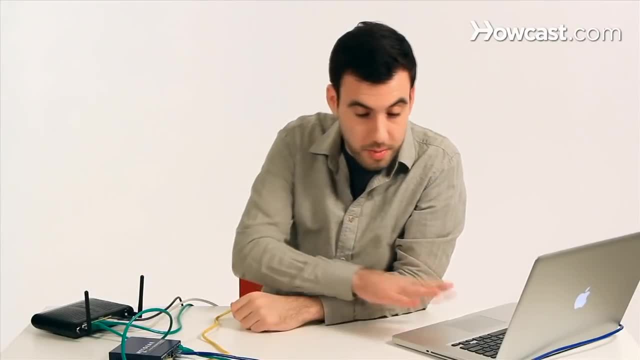 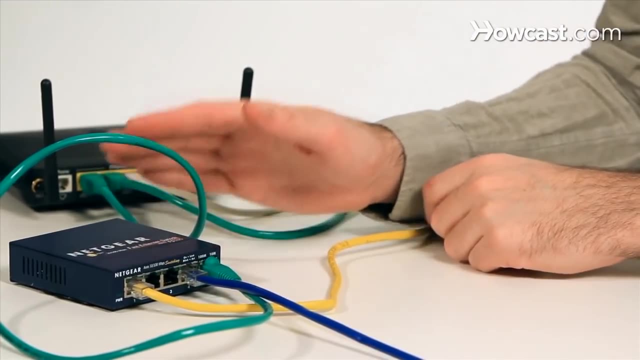 And I'm done, Everybody's online. The laptop is connected to the switch, The switch is connected to the router And everything that's connected to both the router and the switch is on the network. Now, this is a really good trick if you have, for example, another room. 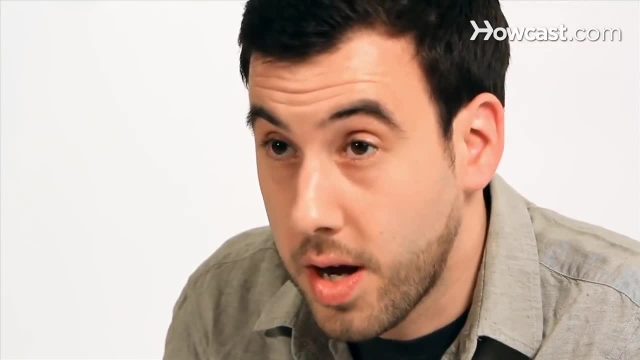 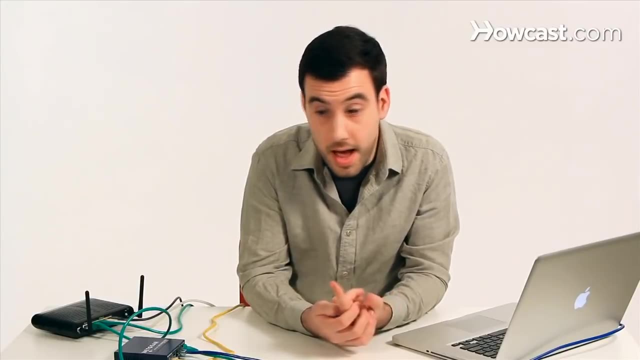 in your house that has a bunch of computers in it that you want to connect to your network, not wirelessly but with an actual cable. This means that you only have to really run one cable over to that room and then just hook it up to a switch that has more ports.